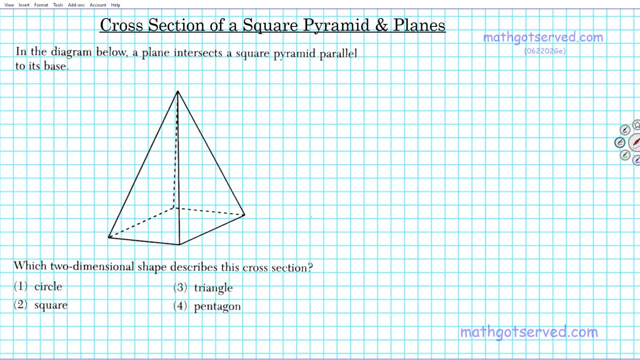 let's go over a very important tip that can help you easily solve problems like this. All right, so here's the tip for solving problems involving pyramids and also um, prisms and cross sections with planes. okay, so this is it right here. if a plane 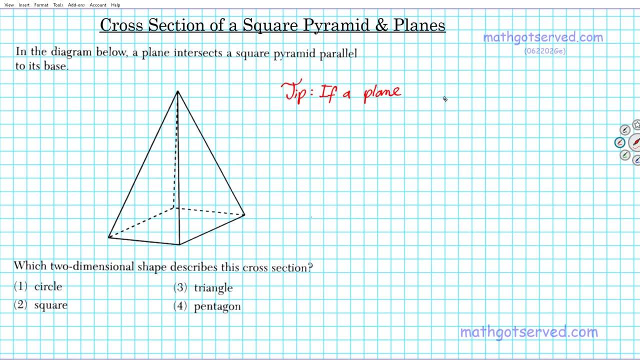 this is like a flat surface, like a piece of paper. all right. intersects a pyramid, as we have in this case. it also applies to prisms too. okay, intersects a pyramid or parallel to its base, all right. the resulting cross section, or the cross section formed, is what the cross section formed is: the shape of the base. okay, this is shape. 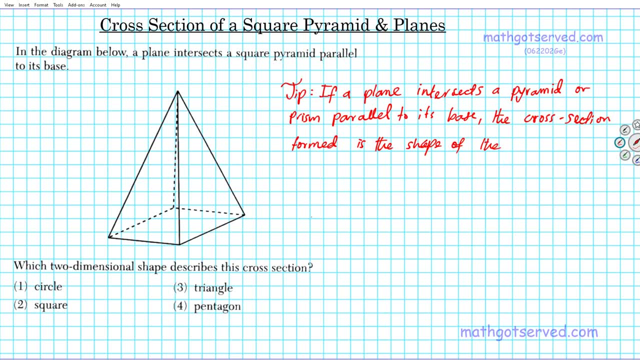 of the base. so what are we saying here? if you take a look at this shape right here, this pyramid, the square pyramid, right, the base is a square. how do we know that the base is a square? because it's a square pyramid. so if you have a plane, intersect this pyramid at any point and it's parallel to this. 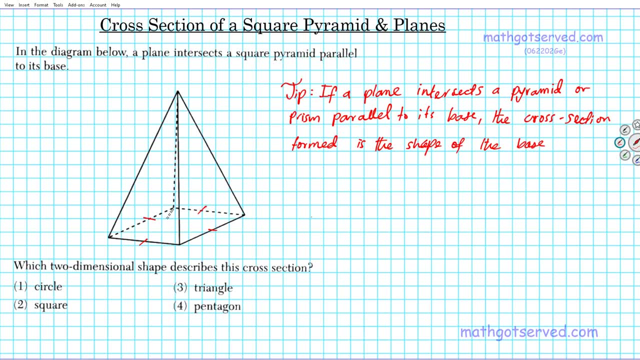 base that the cross section formed will be exactly the shape of the base. all right, so this is the shape of the base. all right, so this is the shape of the base. all right, so this is the shape. Since this is a square pyramid, the resulting shape for the intersection will also be a. 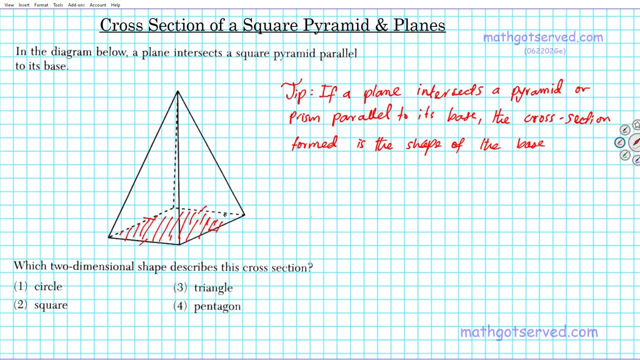 square. Okay, If it were a circular pyramid, the resulting shape would be a circle. If it was a hexagonal pyramid, the same principle holds. It also applies to prisms too. alright, Like right prisms. So let me go ahead and show you a visualization to help you see what we are talking about. 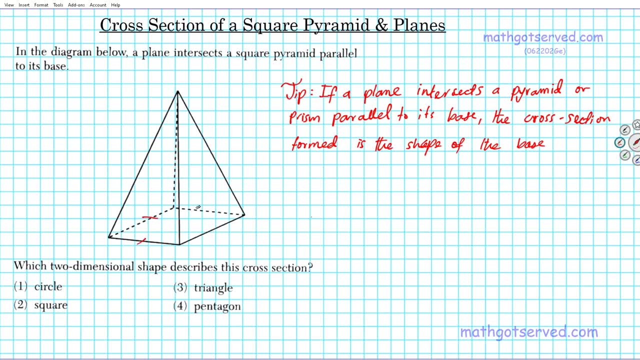 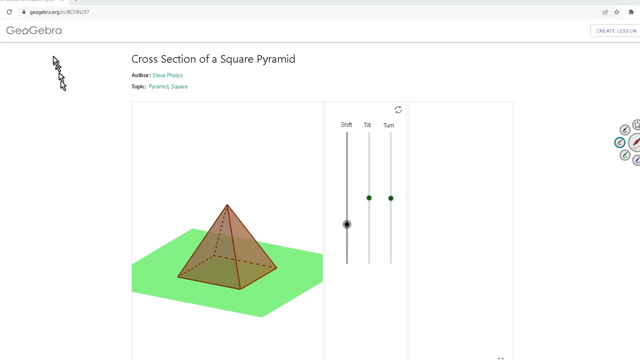 here I'm going to restrict our example to a square pyramid intersected by a parallel, intersected by a plane, Alright, Alright. so here goes a nice little visual right here, created by Steve Phelps. If you want to access this visualization, there goes the URL right there. 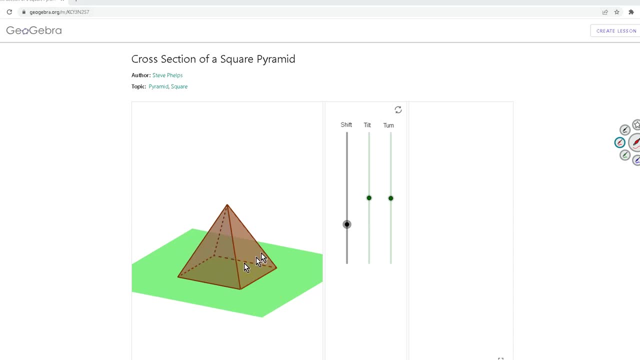 Okay, so here you have a plane and a square pyramid. Alright, so I'm going to. so you see, the plane is at the base, right? So what I'm going to do? What I'm going to do is I'm going to shift the plane upwards into the pyramid and then 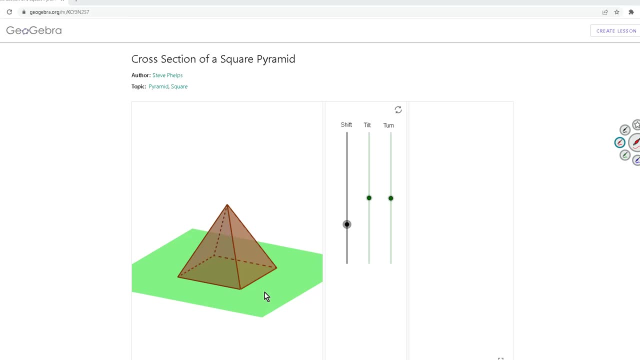 we'll see what kind of cross-sectional shape is created. So I'm going to shift it up. bam, bam, bam. You notice what's happening. It's exactly the same shape as the base, it's just smaller, right until you get to the 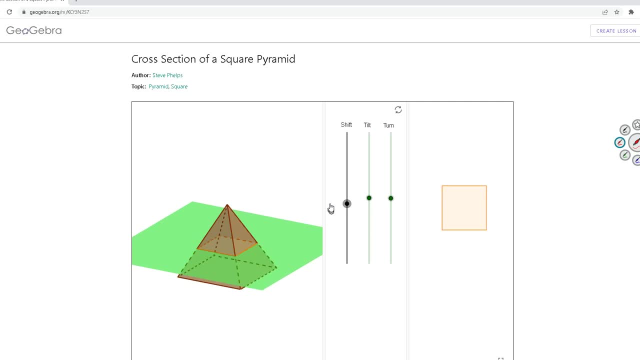 top, then it becomes a point: alright. So this illustrates what we were talking about earlier, which is that if a plane cuts a pyramid parallel to it, Alright. If a plane cuts a pyramid parallel to its base, the shape form, this the cross-section. 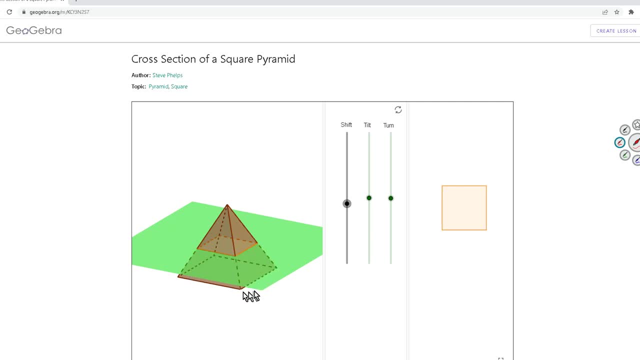 is exactly the same shape as the base shape. Alright, It could be a different size, but it's going to be exactly the same shape. Okay, so you can see the cross-section here is a square, So let's take a look at two other cases, just for your information. 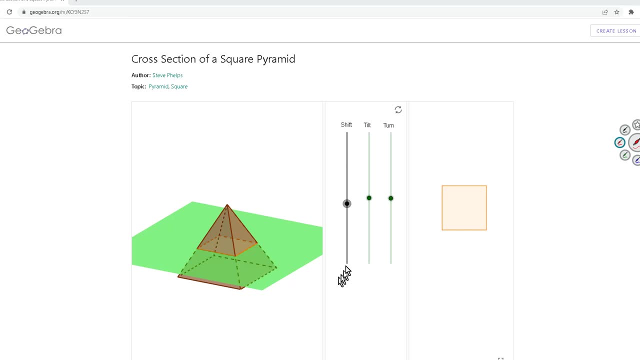 What if the plane is at an angle? Okay, if the plane is tilted like this, okay, it's tilted up. Okay, It's tilted up. Okay, So it's tilted up. What kind of shape does this look like? If the shape is tilted, in certain cases, you can generate a trapezoid. 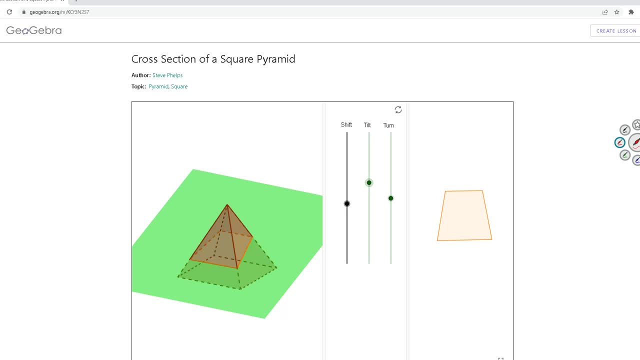 Alright, So you have a trapezoid right here. Now. another case is: what if the plane is perpendicular to the base and goes through the peak or the tip? Okay, Or let's call it the apex. alright, The vertex right here. 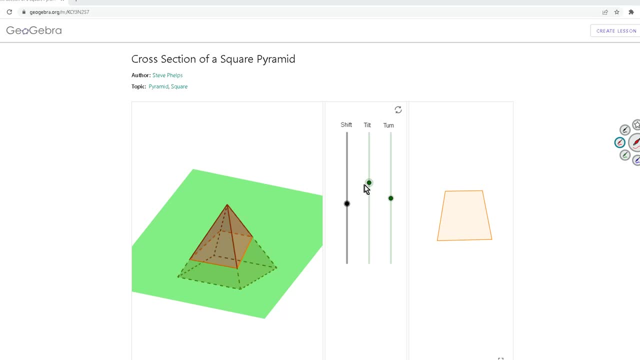 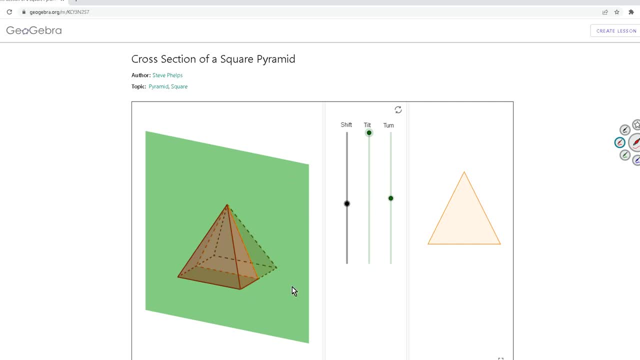 So you have a triangle. So if the plane is perpendicular to the base, through the apex, you have a triangle, Okay. If it's at an angle, you have a trapezoid, alright. And if it's parallel to the base, you have a square. 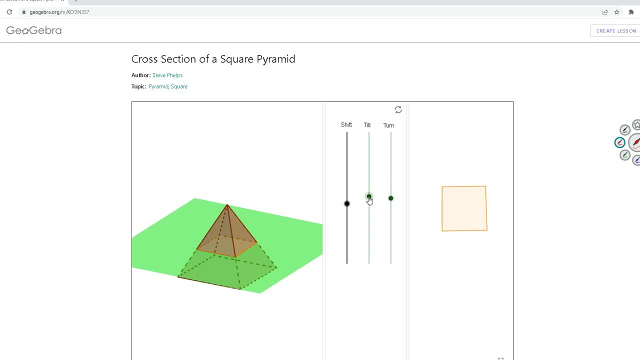 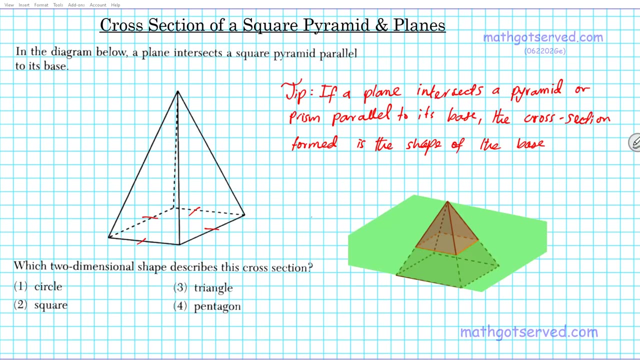 Alright. So different cases, But the one we're looking at is when it's parallel to the base. Okay, so back to the question. We just have a snapshot here of what we're looking at earlier. Now let's go ahead and highlight exactly what the intersection is. alright, 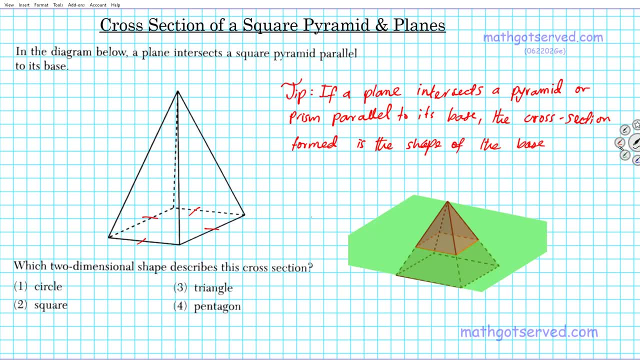 So if you take a look at the intersection, what is it? Do you see? what intersection is? The intersection right here that we're talking about is this outline. Okay, If you slice the pyramid, the square pyramid, what's the outline of that area going to be? 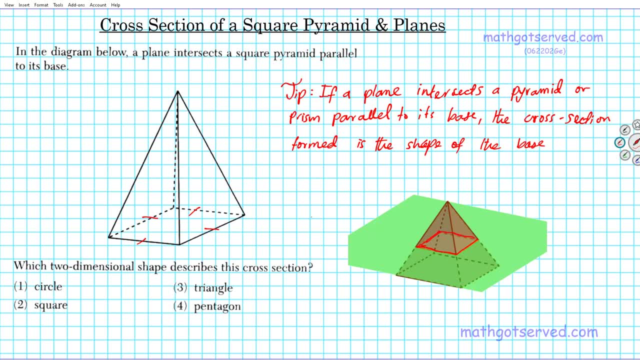 at the point where you slice it. You see right there. That, ladies and gentlemen, is a cross section. Okay, And that shape is a square, The same shape as the base. As long as this plane is parallel to the base, the shape of the cross sectional region is: 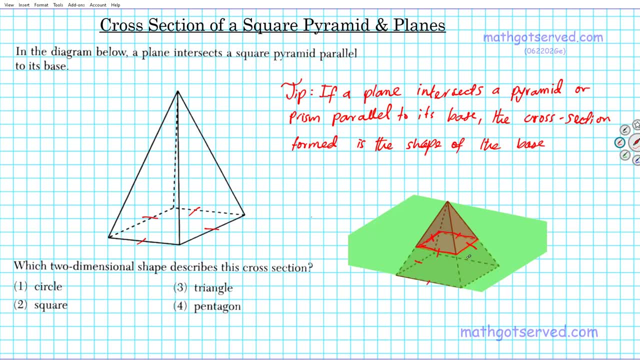 going to be identical to the shape of the base. Okay, It's going to be a smaller size, but it's going to be the same shape, Alright. So this right here. let's go ahead and specify what it is: The cross section. the cross section is a square. 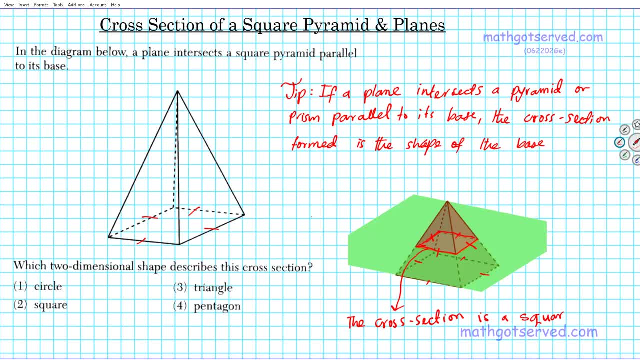 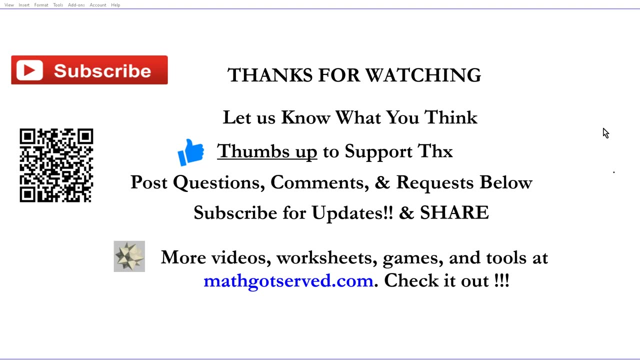 That's the two dimensional resulting shape. Okay, So answer to this question is option number two. Thank you, ائ. Thanks so much for taking the time to watch this presentation. I really appreciate it. Don't forget to support our channel. Tons of support resources can be found on MathGutsServecom. 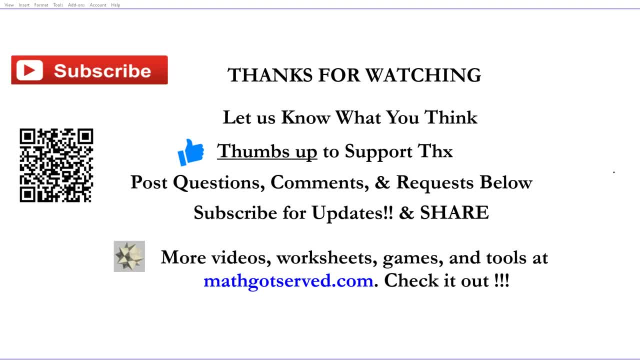 Do check it out. Do let us know what you think about this tutorial. Do you have any special requests? you can specify in the comment section below or just let us know how your day is going. Thanks again for watching and we'll see you in the next video. Goodbye.